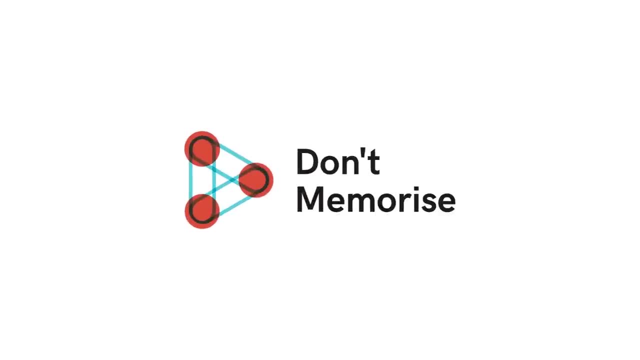 In this video, my aim is to give you the basic understanding of the terms virtual and real images. It's a slightly long video, but it'll be one of the most interesting ones too. I'm sure you'll enjoy it. What you see on your screen is a mirror. 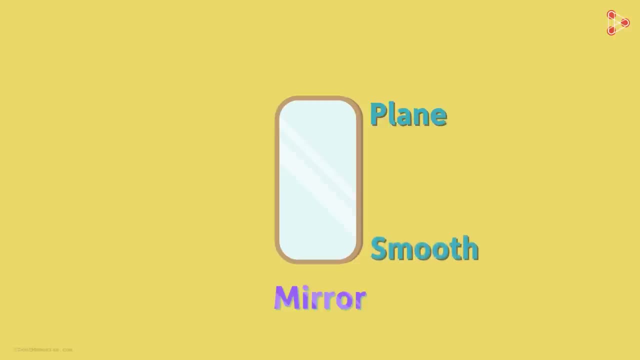 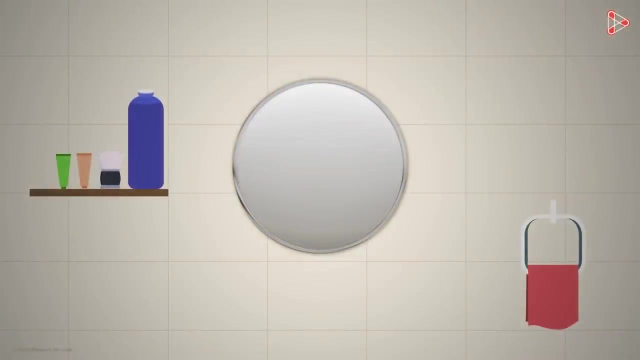 It has this plain and smooth reflecting surface on one side. It's called a plain mirror because its reflecting surface is flat. What other types of mirrors have you seen? Have you seen this type of mirror? Well, you must have seen it on the stand of your bathroom, or maybe hung up there on a 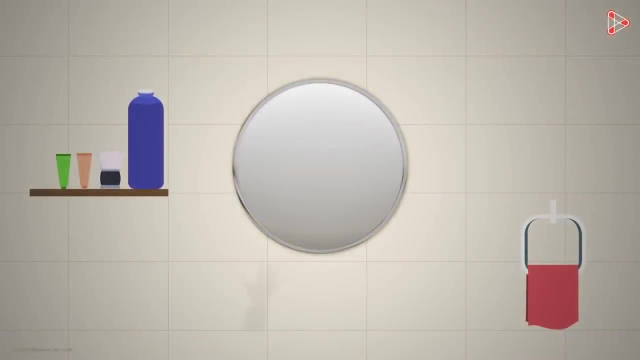 wall. This is not a plain mirror. Try to move your hands over the surface and you will notice it. This is called spherical mirror or more precisely, spherical concave mirror. It is curved inwards. It is kept there as we use it, mostly when we are shaving. 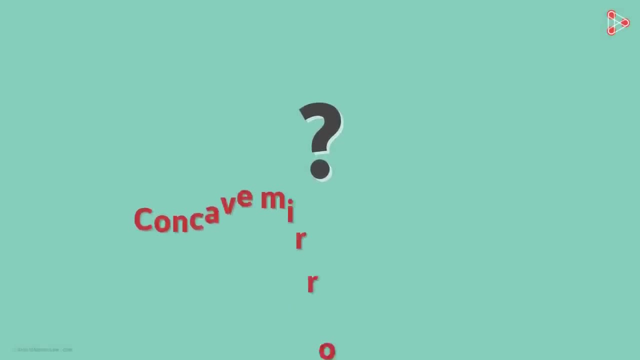 Now the obvious question that must be coming to your mind is: why do we use concave mirror for shaving instead of a plain mirror? For the answer to this question, you have to wait for our future videos. For now, we will be concentrating on the plain mirror only. 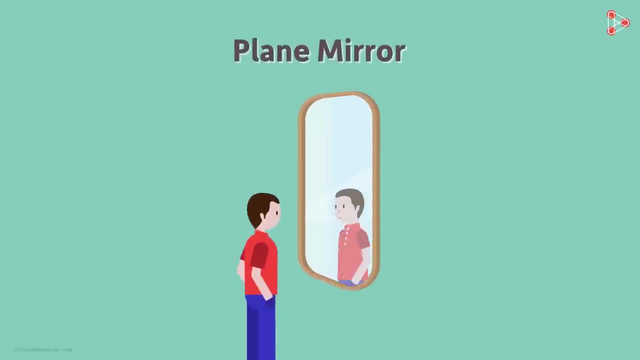 So let's consider this plain mirror again. When we stand in front of a mirror, we see an image of ourselves in the mirror. Nothing surprising there. Why are we able to see our image? Yes, it's due to the reflection of light. 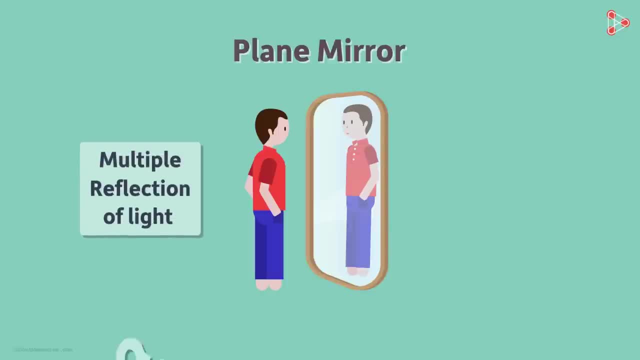 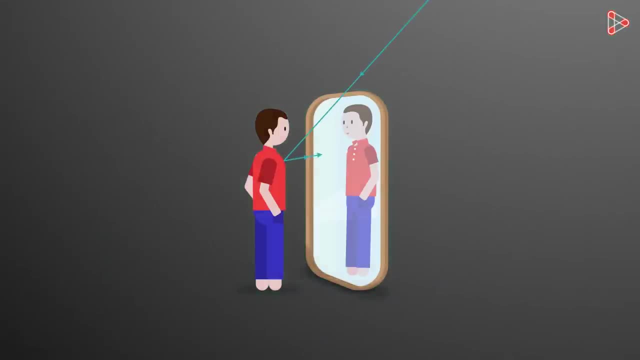 In fact, it's due to multiple reflections of light rays. How The light rays from the source are first incident on our body. They bounce off from our body and fall on the surface of the mirror and again gets reflected from there. This reflected light then reaches our eyes and we see our image. 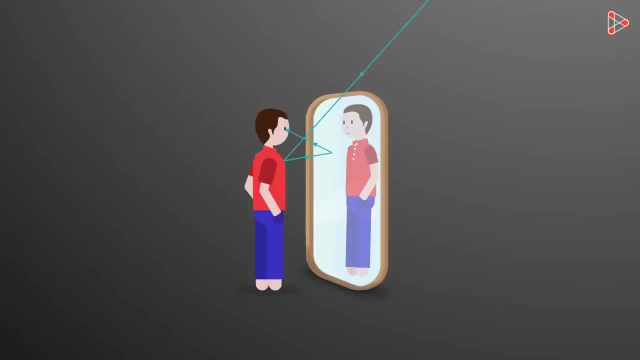 So what does this tell us? Yes, This tells us that a light ray can get reflected multiple times. The same thing happens for every other non-luminous object as well. If you remember, my initial goal was to explain what virtual and real images are. 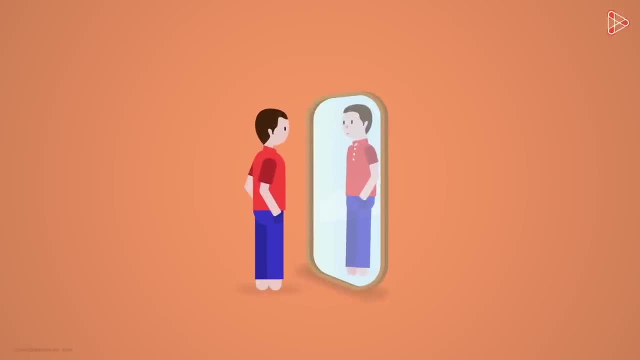 Let me ask you a question: This image that you see here, is it a real image or a virtual one? This image is a virtual image. In order to explain what a virtual image is, let's first simplify it. Let's first simplify it. 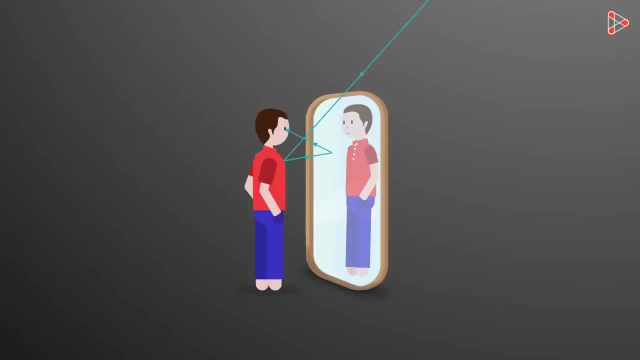 So what does this tell us? Yes, This tells us that a light ray can get reflected multiple times. The same thing happens for every other non-luminous object as well. If you remember, my initial goal was to explain what virtual and real images are. 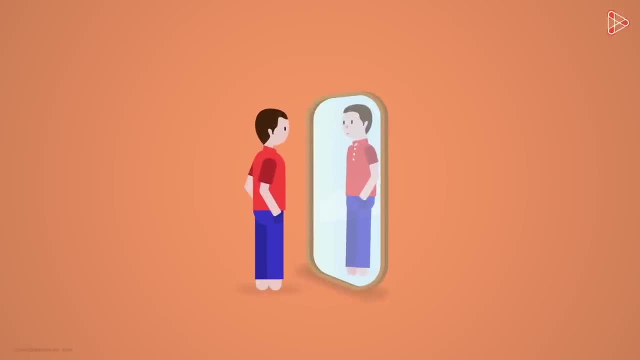 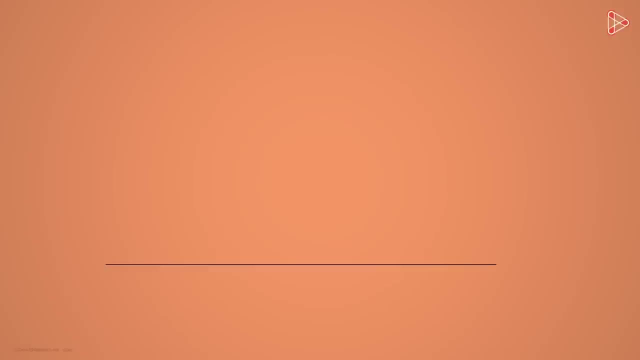 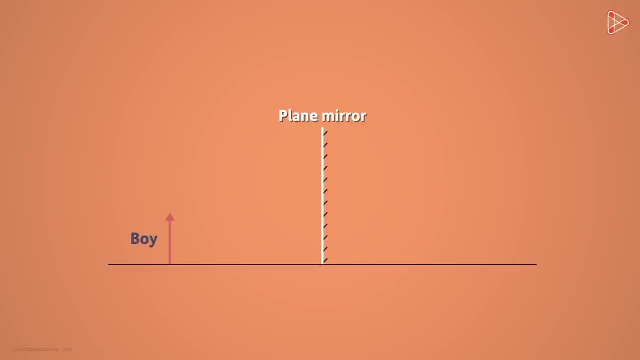 Now, where is the image of the boy formed? When we see the image in the mirror, it seems to us that the image is formed somewhere behind the mirror. But there is nothing behind the mirror. right For us, the light rays seem to come from the location present behind the mirror. 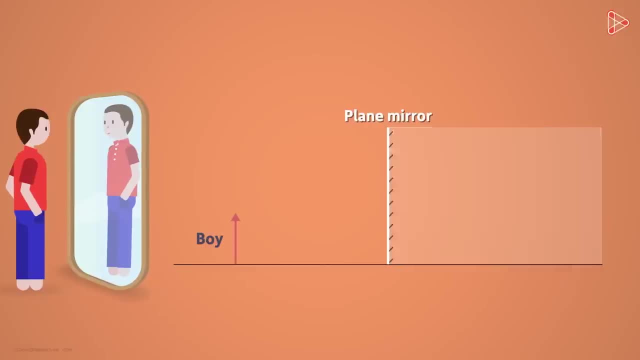 For us, the light rays seem to come from behind the chair. The light rays in the mirror or from the light rays in the mirror are not the same. present behind the mirror, For instance, consider a few light rays emerging from top of the arrow. 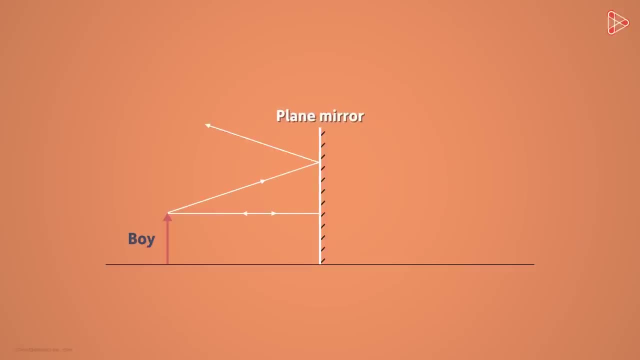 All these rays are incident on the mirror and get reflected back. Yes, all the reflected rays will follow the laws of reflection. You see that all the reflected rays are moving away from each other, ie they are diverging, But we know that the image is formed somewhere behind the mirror. 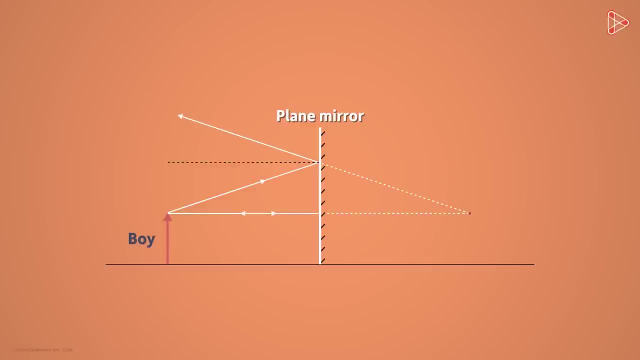 So let me extend these reflected rays backwards and see what happens. We see that they meet at this point, behind the mirror, And to us, this is where the top of the image appears to be. When we look at this point, it appears to us that all the light rays are diverging from. 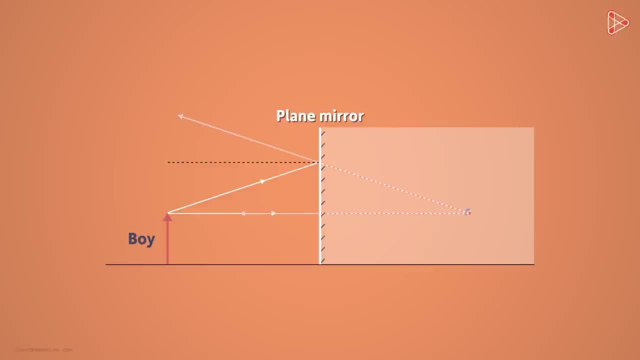 this point, But in reality there are no light rays behind the mirror. This, being a smooth and shiny surface, reflects most of the light back and almost no light reaches behind, But yet we have the perception that the light rays are coming from the point behind. 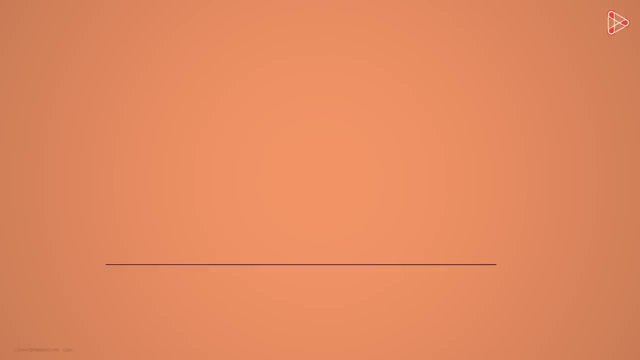 Let's first simplify it. Let's first simplify it. So let's simplify this image. Let's represent this boy with an arrow pointing up. Oh, And here is our plain mirror. You can assume the top of the arrow to be the top of the HEAD of a boy. 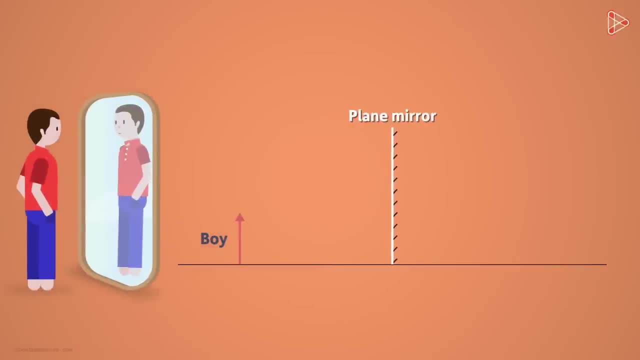 Now, where is the image of the boy formed? When we see the image in the mirror, it seems to us that the image is formed somewhere behind the mirror, But there is nothing BEHIND the mirror, right from the location present behind the mirror. 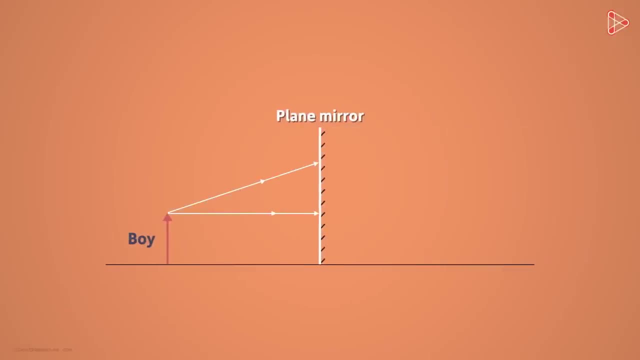 For instance, consider a few light rays emerging from top of the arrow. All these rays are incident on the mirror and get reflected back. Yes, all the reflected rays will follow the laws of reflection. You see that all the reflected rays are moving away from each other, ie they are diverging. 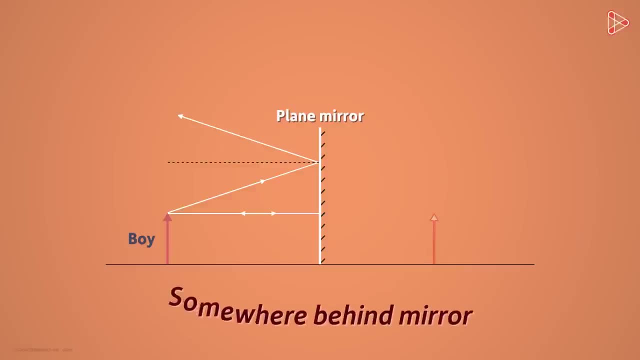 But we know that the image is formed somewhere behind the mirror. So let me extend these reflected rays backwards and see what happens. We see that they meet at this point behind the mirror And to us this is where the top of the image appears to be. 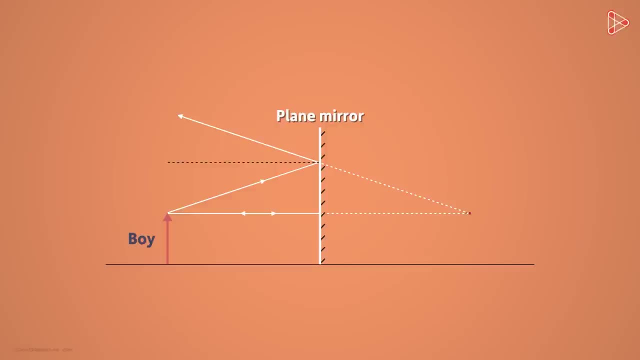 When we look at this point, it appears to us that all the light rays are diverging from this point, But in reality there are no light rays behind the mirror. This, being a smooth and shiny surface, reflects most of the light back and almost no light. 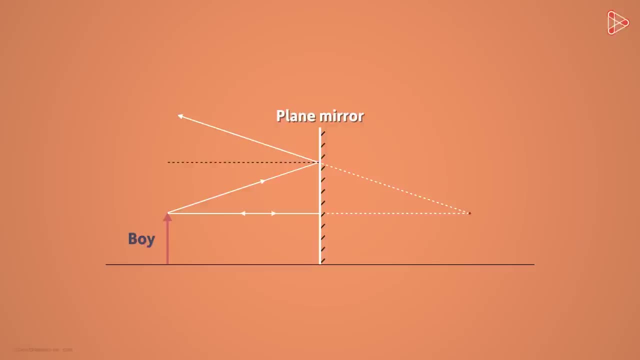 reaches behind, But yet we have the perception that the light rays are coming from the point behind. So we just consider the top of the arrow here. We can do something similar for the remaining points on the object to get the complete image. So we say that the image formed here is virtual, or in other words not real. 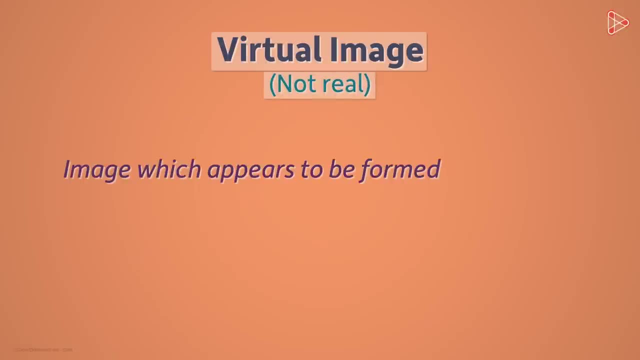 You can think of a virtual image as an image which appears to be formed in a position somewhere behind the mirror, But in reality it isn't there. A virtual image is formed when the light rays diverge after reflection from the mirror. Every plane mirror forms a virtual image. 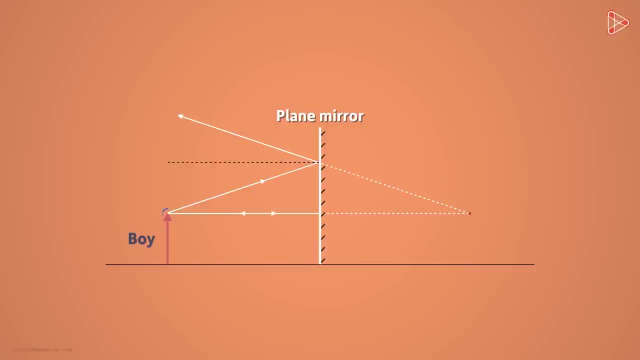 So we just consider the top of the arrow here. We can do something similar for the remaining points on the object to get the complete image. So we say that the image formed here is virtual, or in other words not real. You can think of a virtual image as an image which appears to be formed in a position, somewhere. 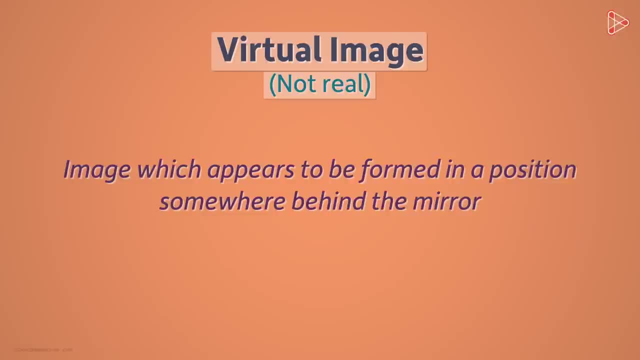 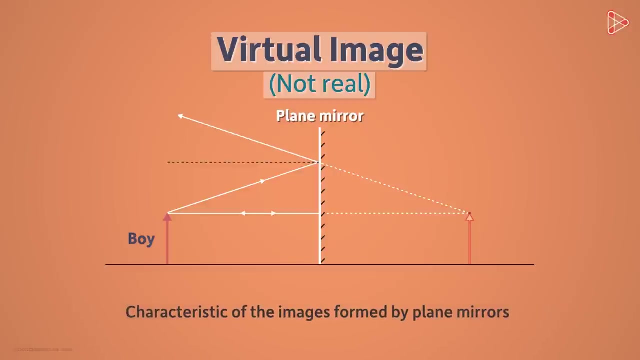 behind the mirror, But in reality it isn't there. A virtual image is formed when the light rays diverge after reflection from the mirror. Every plane mirror forms a virtual image. This is the first characteristic of the images formed by plane mirrors. 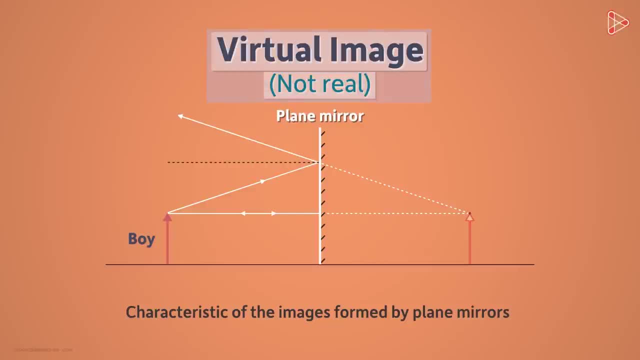 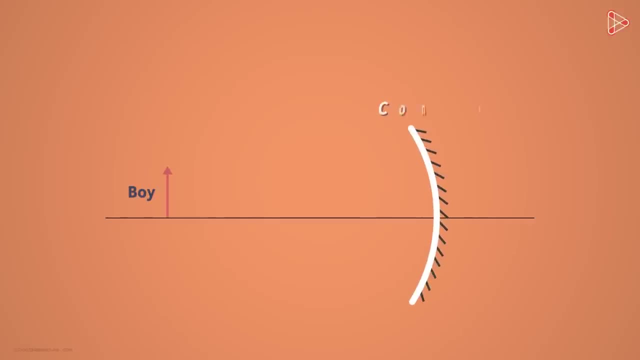 Images formed by plane mirrors are virtual and not real. So what is the real image then, and how are they formed? Let's replace this plane mirror with a spherical concave mirror. Why? Because real images can be formed by concave mirrors. Let's consider the light rays from the same point of the object incident on the mirror. 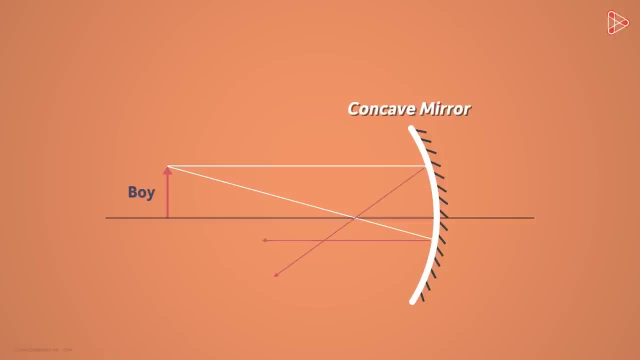 We see that after reflection, each ray is travelling in a certain direction. Note that here as well, each ray obeys the law of reflection. What difference did you notice here compared to the plane mirror reflection? In the previous case, all the reflected rays were diverging. 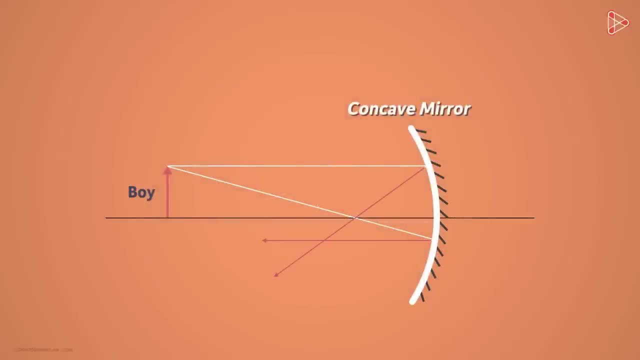 Yes, Here all the reflected rays after reflection are intersecting each other at this point, or we can say that they are converging at this point And the image of the top of the arrow is formed at this point, And we can do something similar for the remaining points of the object too. 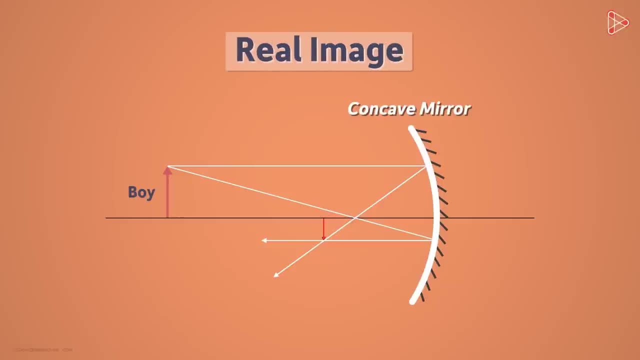 We get this image. This is called a real image. It is the image formed when light rays converge after reflection from the surface. One important thing we need to know is that light rays are converging at this point. This is called a real image. 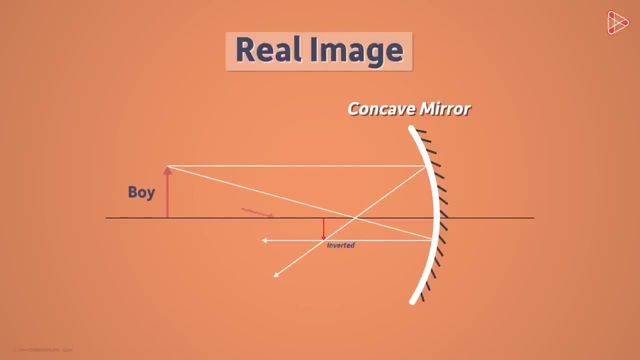 This means that real images formed by concave mirrors are always inverted. We will learn more about this in the future videos. You see that in this case, the image is formed on the same side of the mirror as the object is. Real images are always formed on the same side as that of the object. 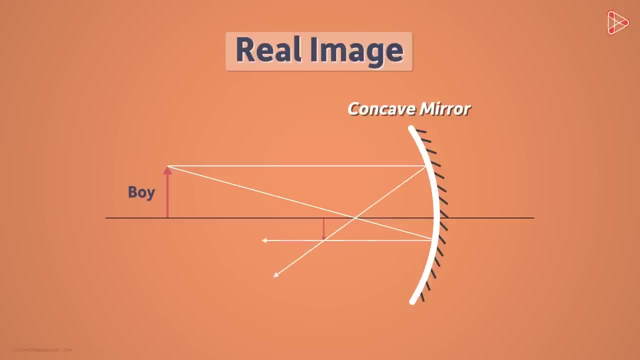 And light rays do reach this position. When we look at the real image formed by a concave mirror, it also seems to us that the light rays are diverging, But here the rays actually are diverging from a point in front of a mirror. 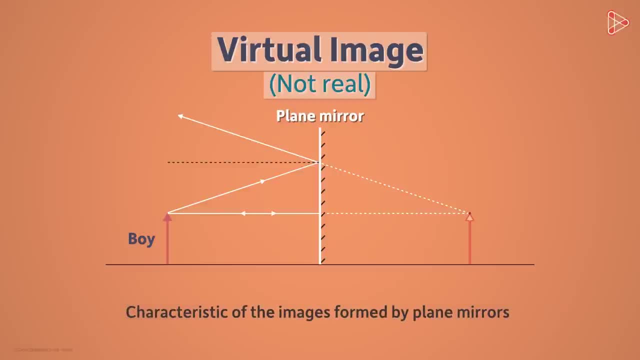 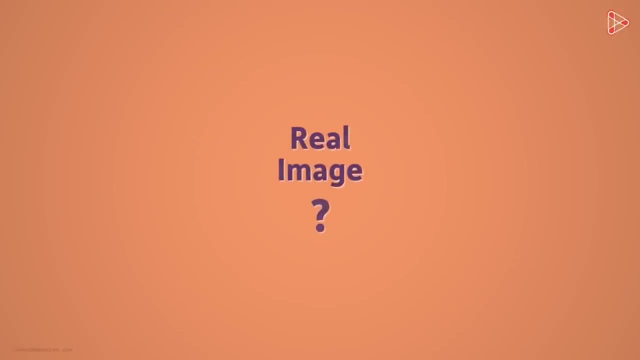 This is the first characteristic of the images formed by plane mirrors. Images formed by plane mirrors are virtual and not real. So what is the real image then, and how are they formed? Let's replace this plane mirror with a spherical concave mirror. Why? 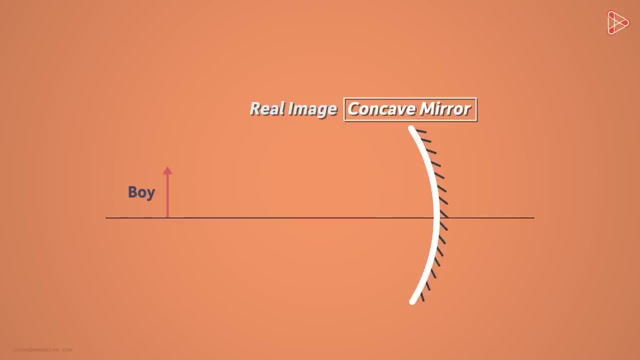 Because real images can be formed by concave mirrors. Let's consider the light rays from the same point of the object incident on the mirror. We see that after reflection, each ray is travelling in a certain direction. Note that here as well, each ray obeys the law of reflection. 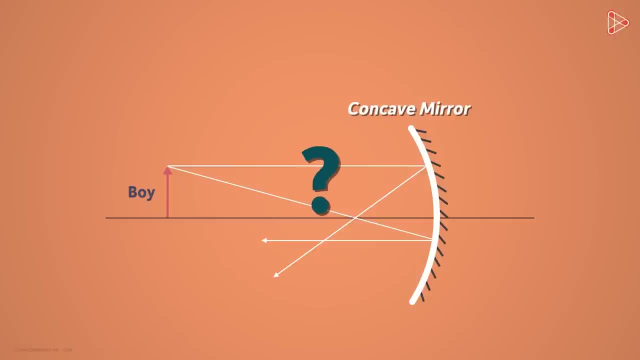 What difference did you notice here compared to the plane mirror reflection? In the previous case, all the reflected rays were diverging. Yes, here all the reflected rays, after reflection, are intersecting each other at this point, or we can say that they are converging at this point. 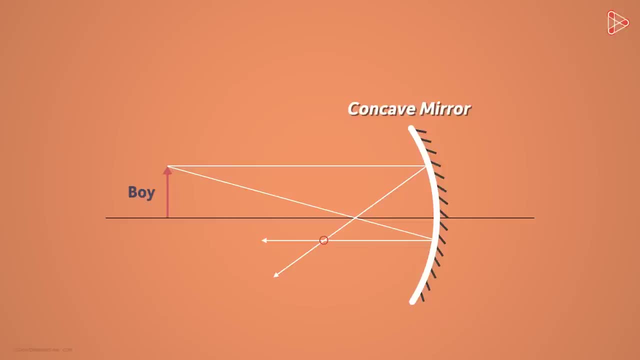 And the image of the top of the arrow is formed at this point, And we can do something similar for the remaining points of the object too. We get this image. This is called a real image. It is the image formed when light rays converge after reflection from the surface. 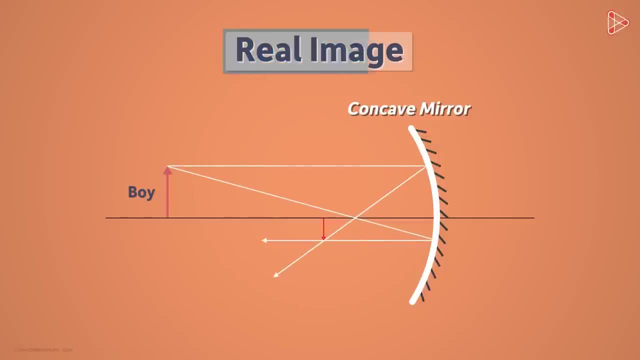 Let's see what happens. One important thing we need to know is that real images formed by concave mirrors are always inverted. We will learn more about this in the future videos. You see that in this case, the image is formed on the same side of the mirror as the object. 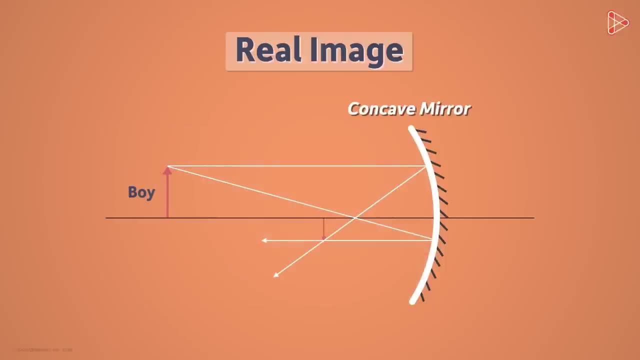 is Real. images are always formed on the same side as that of the object, And light rays do reach this position. When we look at the real image formed by a concave mirror, it also seems to us to be a concave mirror. 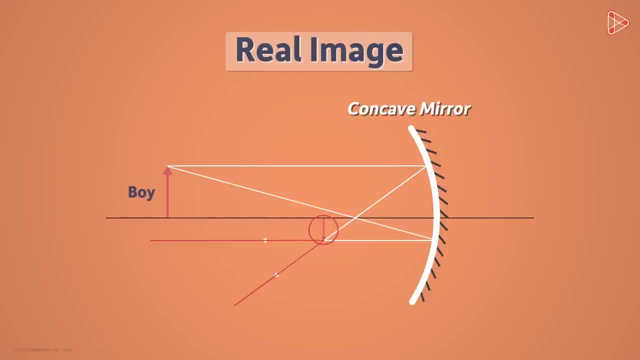 It appears to us that the light rays are diverging, But here the rays actually are diverging from a point in front of a mirror, Whereas in the case of a plain mirror, it appears to us that the rays were diverging from the point behind the mirror. 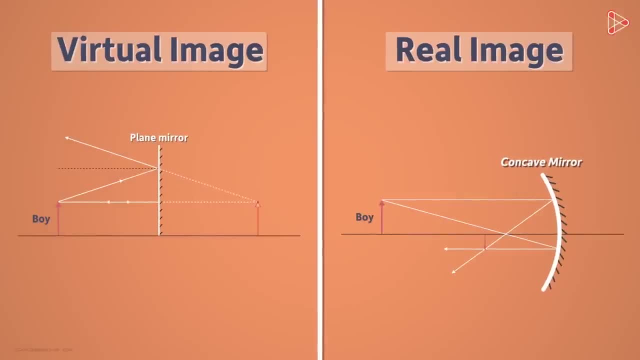 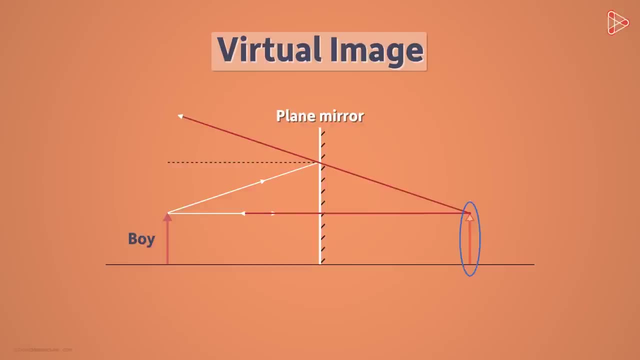 So did you understand the difference between a virtual image and a real image? When we look at a virtual image, it appears to us that the light rays are diverging from a point somewhere behind the mirror, but in reality they aren't, as no light reaches.